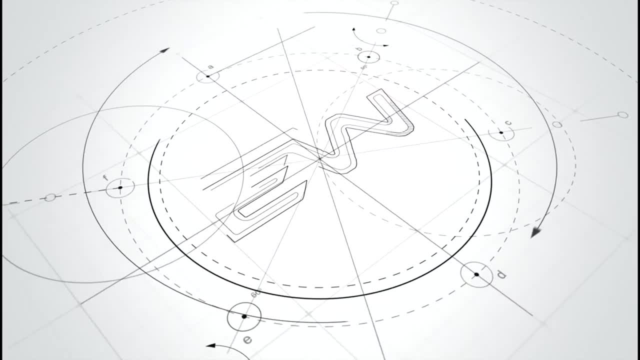 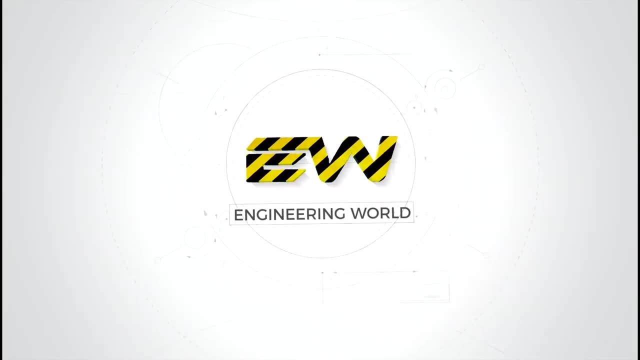 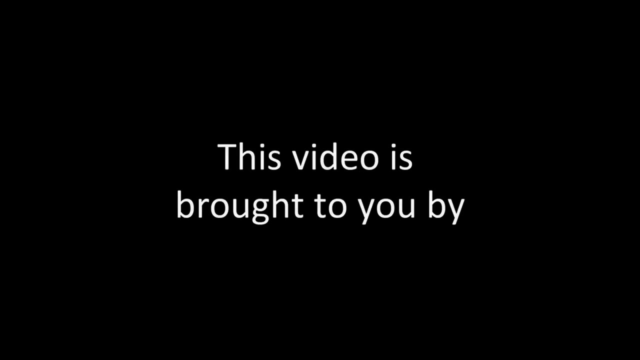 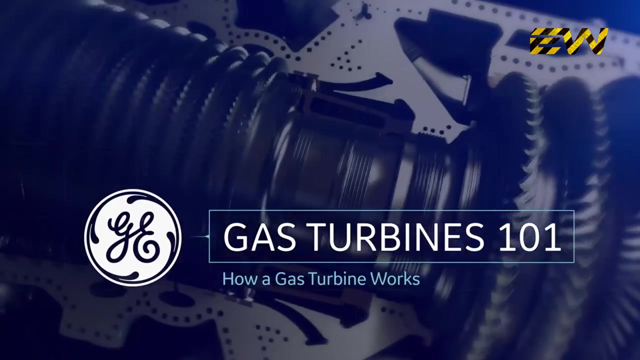 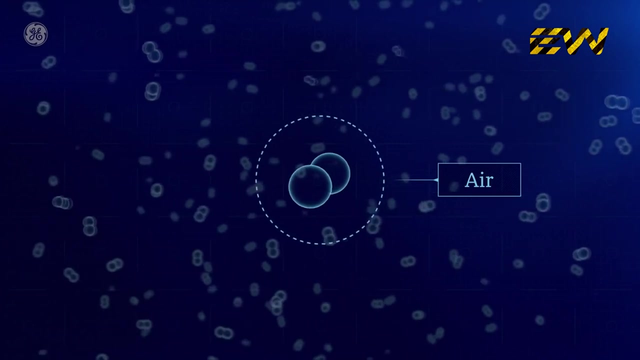 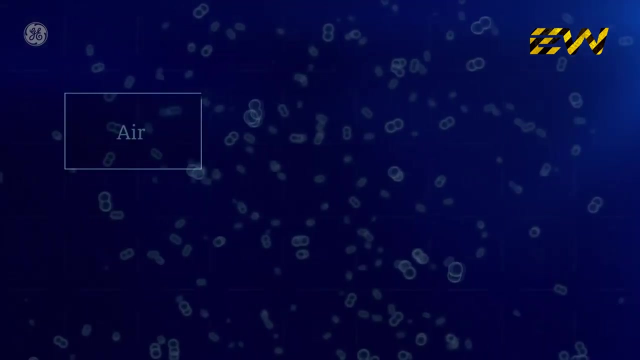 Thank you for watching. Ah air- A lot of gaseous molecules floating all around us. It's great for breathing and, it turns out, it's great for getting lights turned on. That's because air, along with abundant natural gas or other fuels, are the ingredients that combine in a gas turbine. 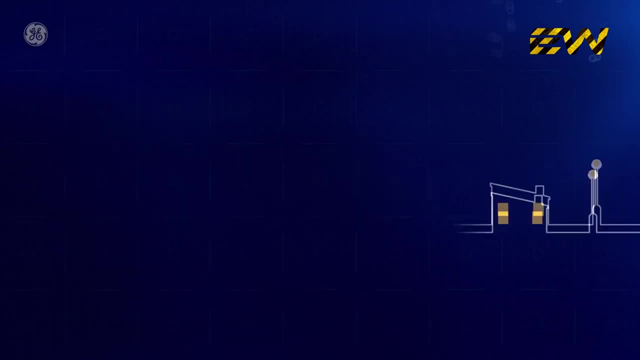 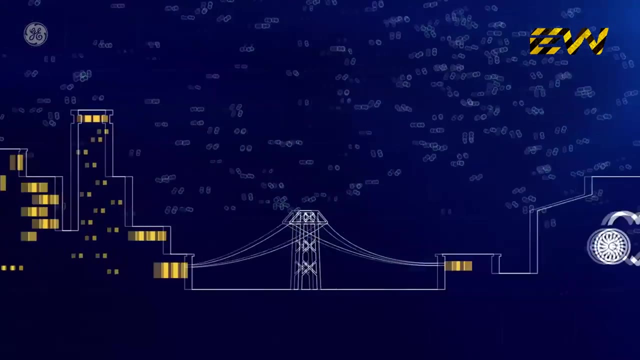 to spin the generator that produces electric current. If you follow the electricity you use at home or at work back through the power lines to your local power plant, you'll see that the process most likely starts with the work of the gas turbine, the very 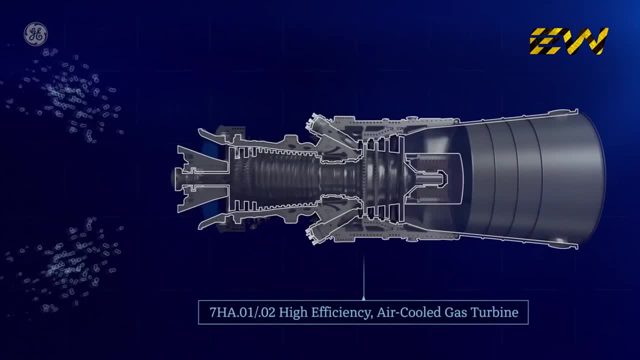 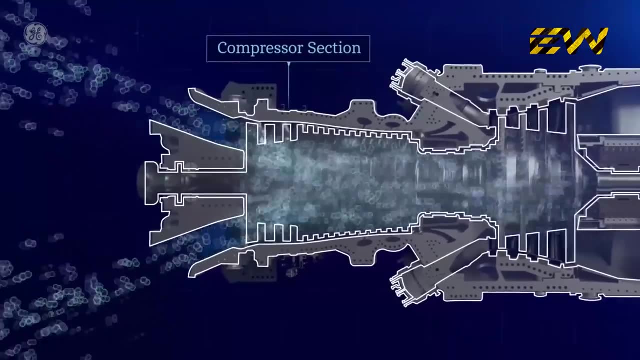 heart of the power plant. First air is drawn in through one end of the turbine. In the compressor section of the turbine all those air molecules are squeezed together, similar to a bicycle pump squeezing air into a tire. As the air is squeezed, it gets hotter and 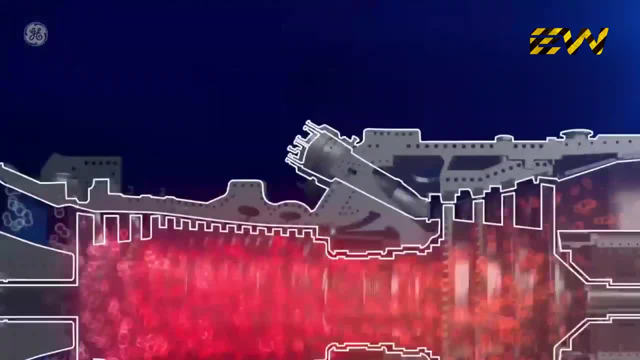 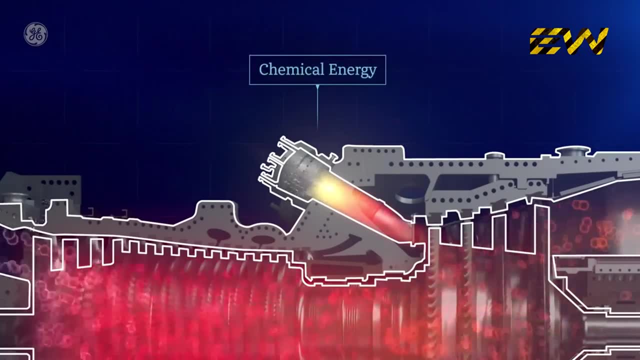 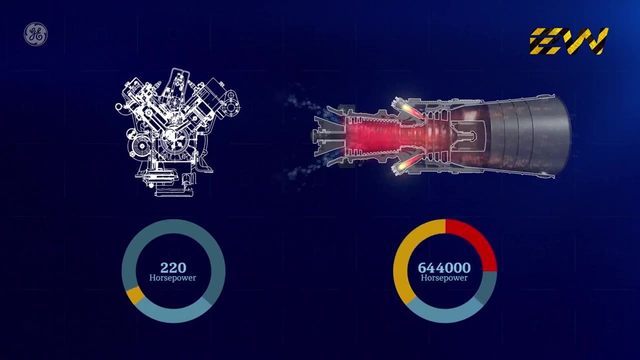 the pressure increases. Next, fuel is injected into the combustor, where it mixes with the hot compressed air and is burned. This is chemical energy at work. Essentially, this is what happens in your family car's engine, but at about 2,900 times more power. Actually, it's exactly like the turbine engines. 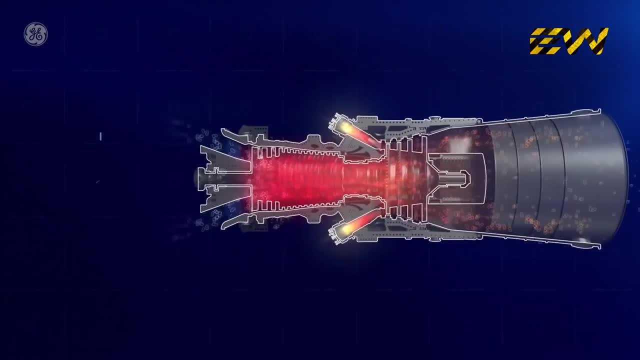 on jet airplanes. The hot gas created from the ignited mixture moves through the turbine blades, forcing them to spin at more than 3,000 RPMs. Chemical energy has now been converted into mechanical energy. The turbine then captures energy from the expanding gas. 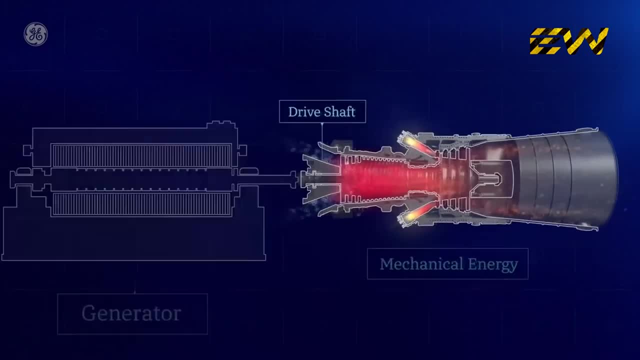 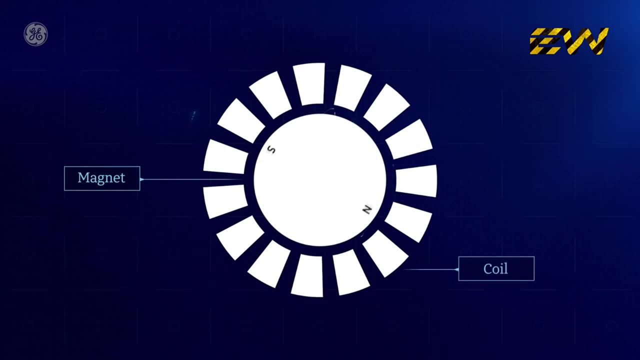 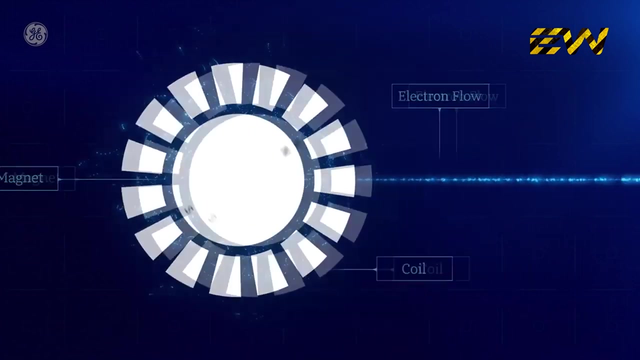 which causes the drive shaft, which is connected to the generator, to rotate. That generator has a large magnet surrounded by coils of copper wire. When that magnet gets rotating fast, it creates a powerful magnetic field that lines up electrons around the coils and causes them to move. The rotating mechanical energy has now been converted into electrical.